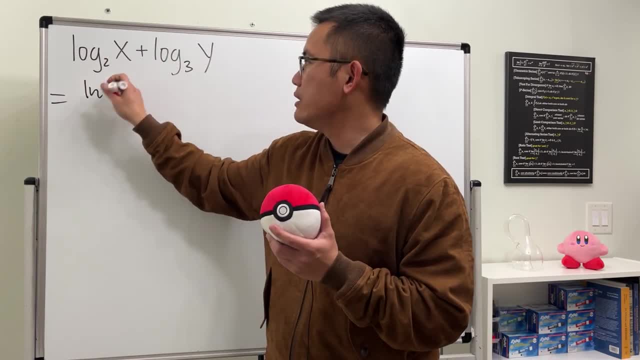 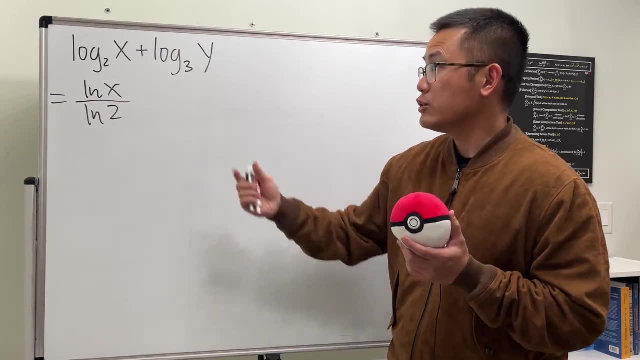 natural log. So we are going to get ln of x over ln of 2.. And again, that's by the change of base formula, And let's do the same thing for the other one. So we are going to add ln y over ln 3.. 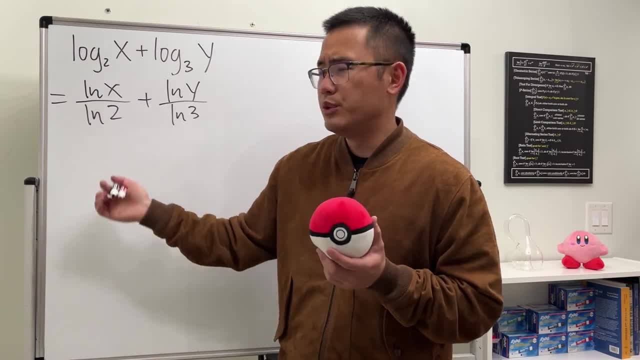 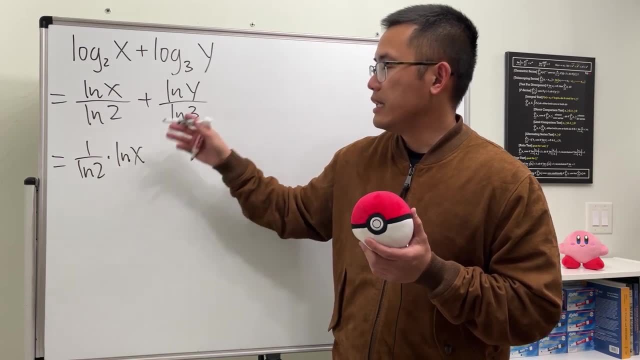 And now let's see we have ln 2 on the button, but that's really the same as saying 1 over ln 2 times ln x. And then let's do the same thing for the second one We are going to add. 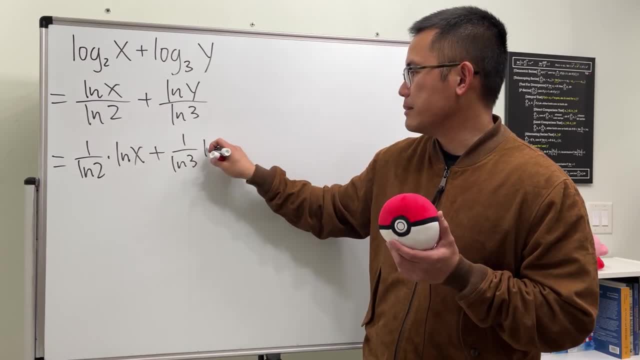 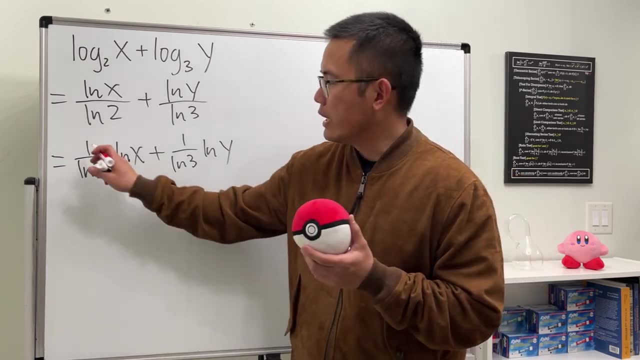 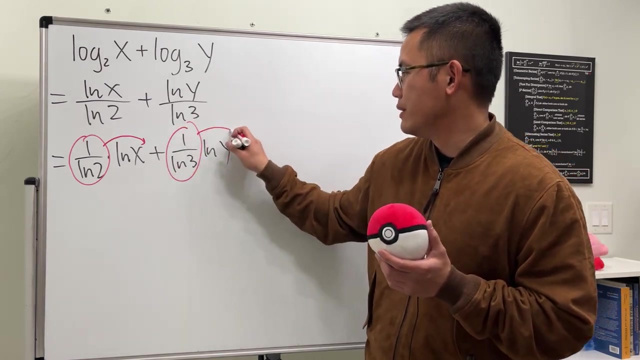 1 over ln, 3 times ln y. And now do we see it? Yeah, right, Because 1 over ln 2 is just a number, So we can actually put this to here and make that into an exponent, And of course, we can do the same thing right here. Aha, So for the first one. 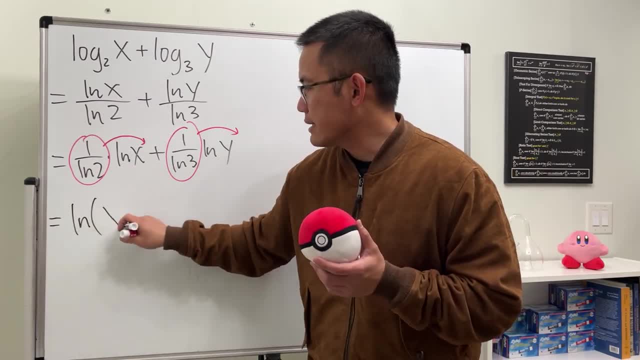 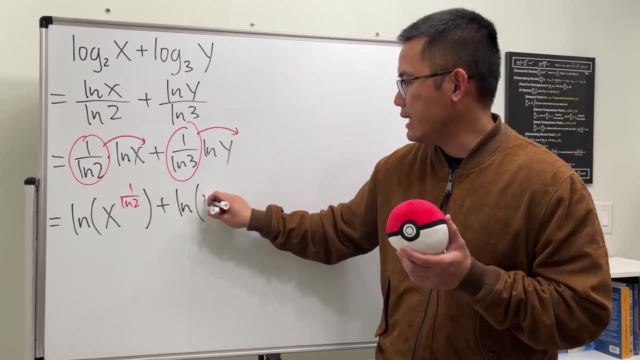 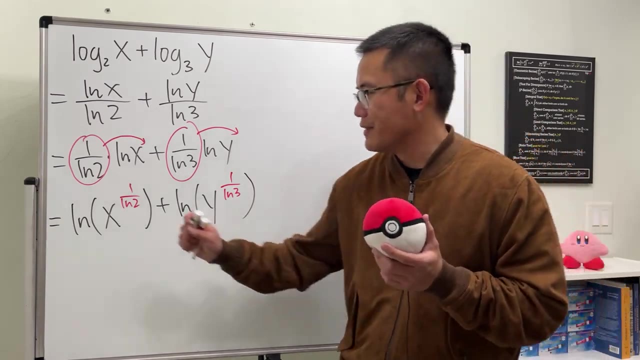 we are really just going to get ln of x to the 1 over ln 2 power, And then we are adding this with ln of y raised to the 1 over ln 3 power. Congratulations, Now we have ln and ln and we are adding, So we can just put the insights together and multiply. 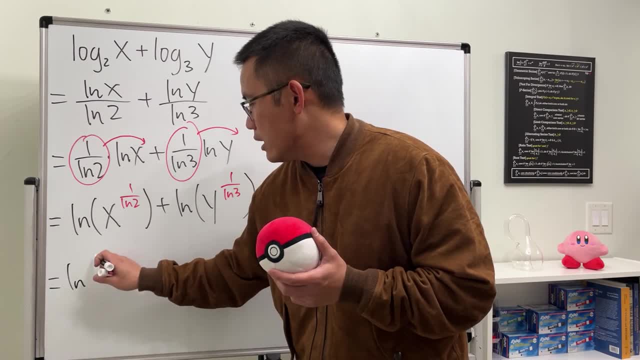 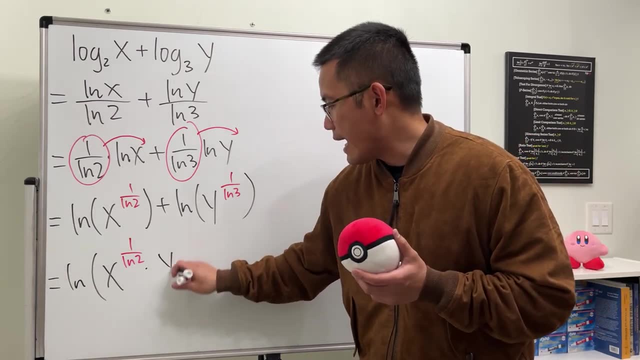 them. So this right here is equal to ln of the first one, which is x to the 1 over ln 2 power, And we multiply this by y raised to the 1 over ln 3 power. So yeah, we just combine. 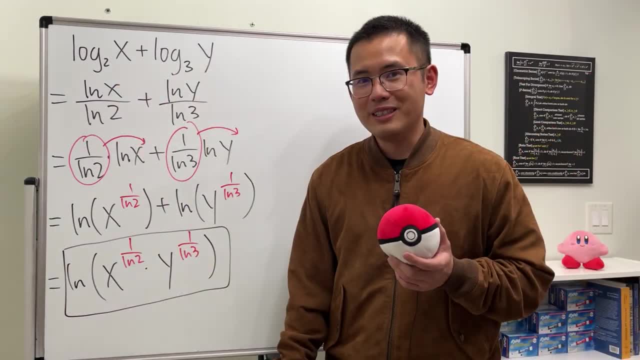 these two logarithms, even though they have different bases. What do you guys think?